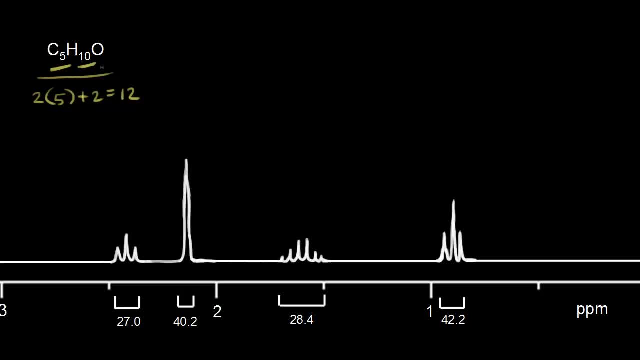 so we're missing two hydrogens. We're missing one pair of hydrogens, and so therefore, the hydrogen deficiency index is equal to one. Immediately, that makes me think about a double bond might be present in this molecule, or one ring. Let's go down to the integration value. 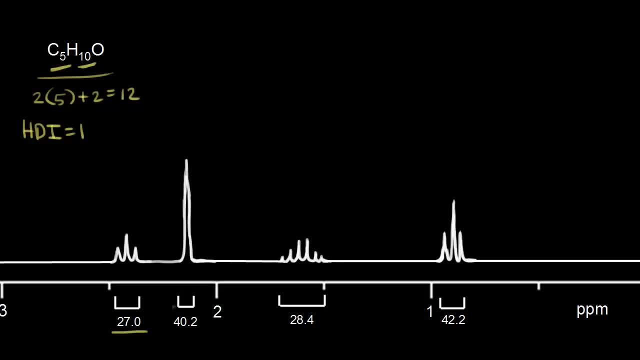 So for this signal there's an integration value of 27.. For this signal, the integration value is 40.2.. For this signal it's 28.4.. And for this signal it's 42.2.. Remember what you do. 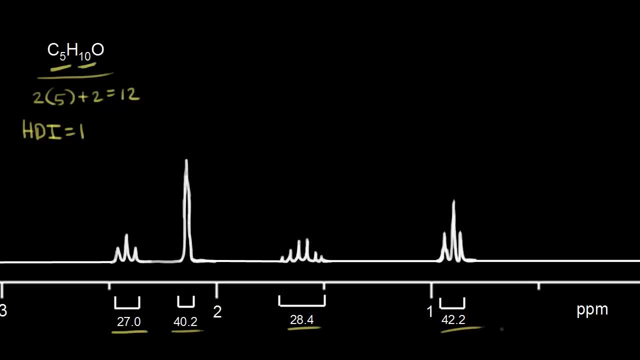 You divide all four integration values by the lowest one, So the lowest one is of course 27.. So 27 divided by 27 is of course one. 40.2 divided by 27 is pretty close to 1.5.. 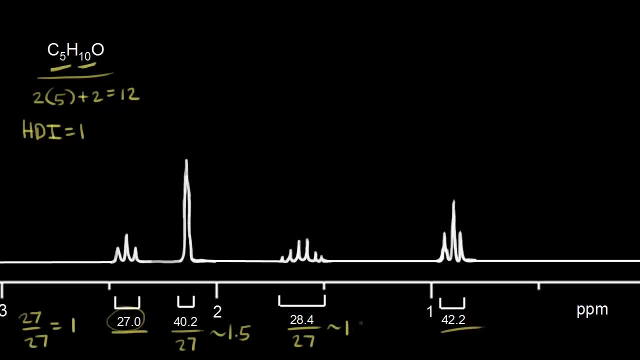 28.4 divided by 27,, that's pretty close to one. And 42.2 divided by 27 is once again pretty close to 1.5.. Remember, these are just the relative numbers of protons giving you these signals. 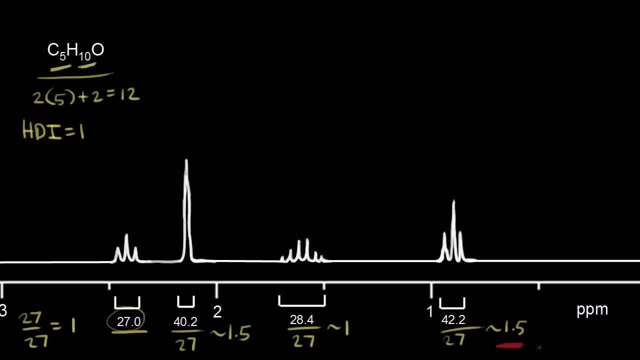 but you can't have 1.5 protons giving you a signal. We need a whole number and we need to account for 10 total protons here. So if we multiply one by two, then we get two protons. So this signal represents two protons. 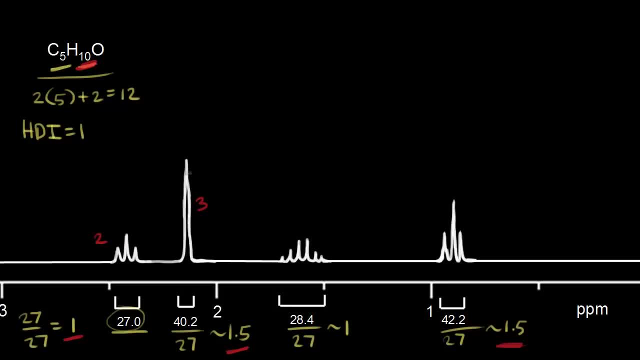 If we multiply 1.5 by two, we get three. So this signal represents three protons. If we multiply one by two, we get two, And if we multiply 1.5 by two, we get three. So if you add all those up, 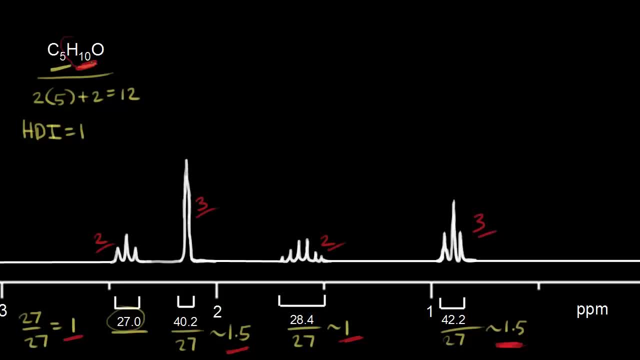 two plus three plus two plus three, that's, of course, 10 protons. So now we've accounted for all 10 protons using our integration values. Next let's look at each signal one by one. So we'll start with this signal. 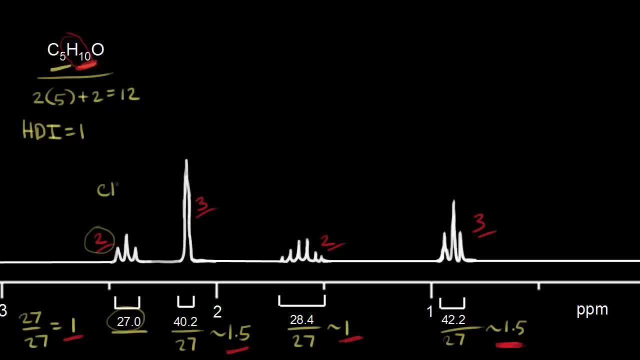 So we have a CH2, since we have two protons, So this signal represents a CH2.. How many neighboring protons do those CH2 protons have? So we can figure that out by the number of peaks on the signal. So this signal here has one, two, three peaks. 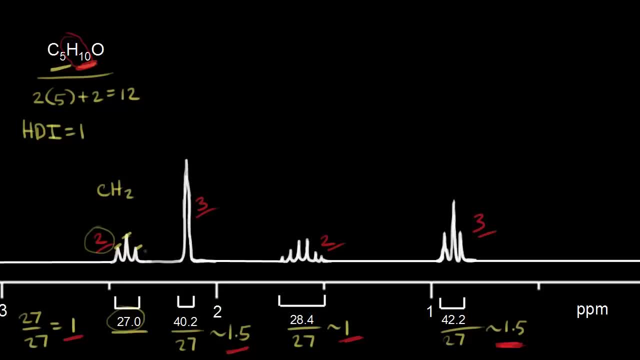 And if you think about the n plus one rule, if you have n neighbors you get n plus one peaks. So if we have three peaks, all we have to do is subtract one to find out how many neighboring protons. So three minus one is equal to two. 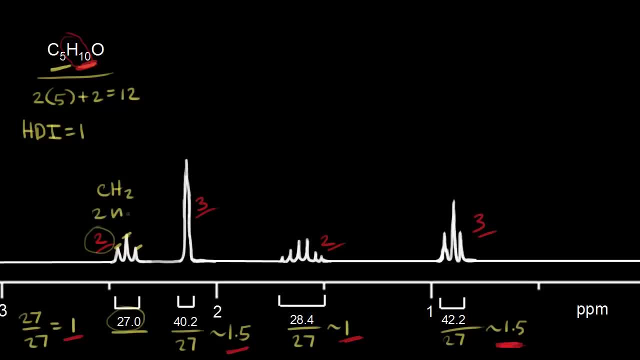 So this CH2, these CH2 protons have two neighboring protons. Let's think about the chemical shift for this signal. So the chemical shift for this signal is between two parts per million and 2.5.. And that's in the region for a proton. 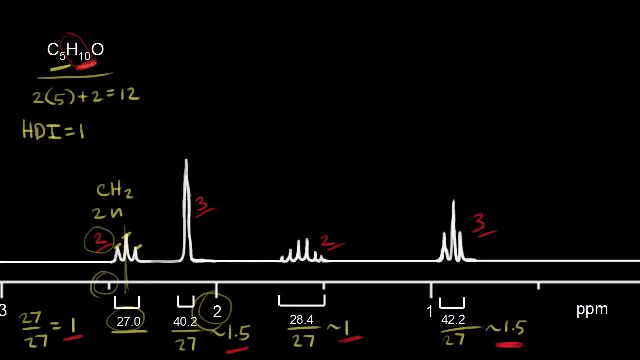 next to a carbonyl. And that would make a lot of sense because we calculated an HDI of one indicating there might be a double bond present, And we need to account for an oxygen in our molecular formula. So let's go ahead and draw in a carbonyl. 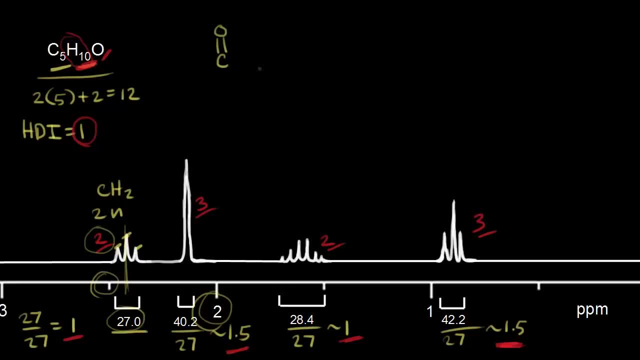 And these CH2 protons are next to the carbonyl. We know that because of the shift right The carbonyl, the oxygen, deshields these two protons a little bit and gives us a higher value for the chemical shift. 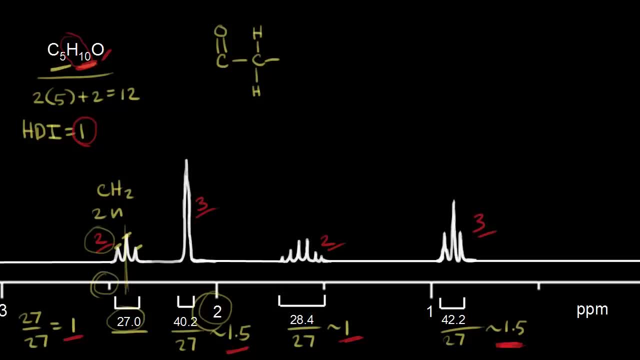 compared to something in an alkane type region. All right, let's color these protons in here magenta. So we're saying this signal is due to those two protons. Let's move on to the next signal. So we have three protons. 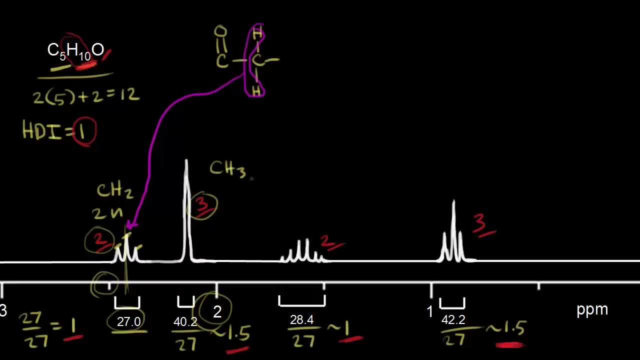 That would be a methyl group, so CH3.. How many neighboring protons? for those methyl protons? Well, there's only one peak here. So one minus one is zero. So zero neighboring protons. What about the chemical shift? So the chemical shift for this signal. 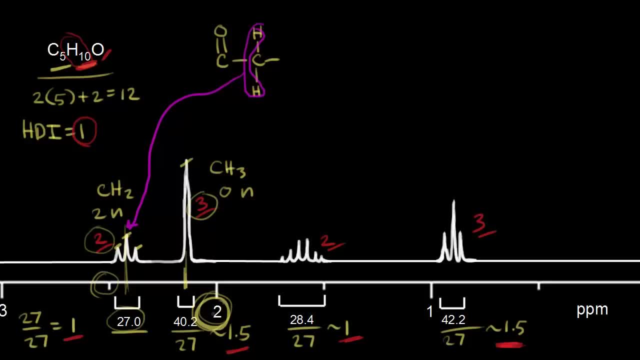 is once again past two parts per million. So this signal is deshielded, right. So these protons must be deshielded a little bit And those must be next to our carbonyl. So we'll draw in our methyl protons, right? 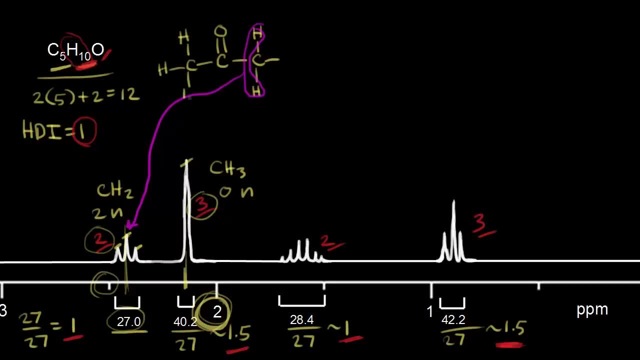 Being deshielded Because they're next to the carbonyl. And let's make these blue. So these protons in blue here, These three protons, are giving us this signal And we should expect zero neighboring protons. All right, so those protons are on this carbon. 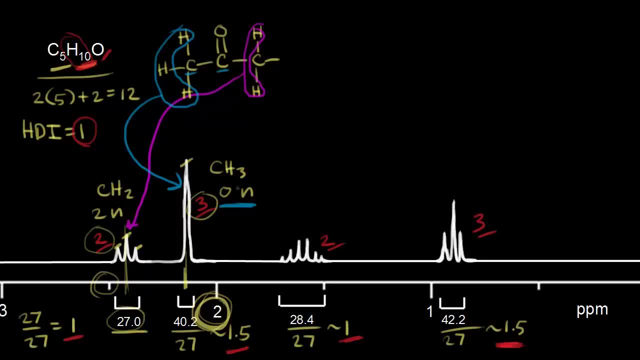 And the next door. carbon has no protons on it, So zero neighboring protons makes sense. Move on to the next signal. So this signal represents two protons, So that's a CH2.. How many neighboring protons? All right? well, let's count up how many peaks we have. 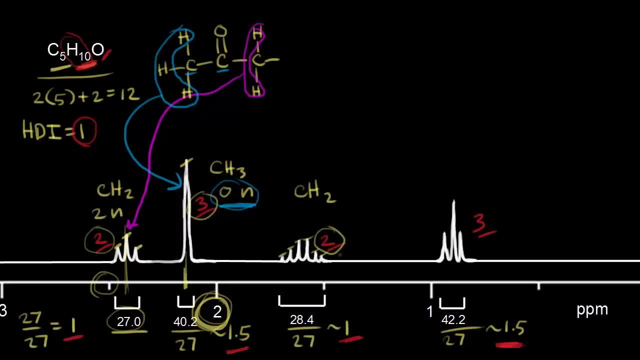 One, two, three, four, five, six, So six peaks. So we subtract one from that, So six minus one is five. So we would expect five neighboring protons. Let's move on to the next signal. Three protons right. 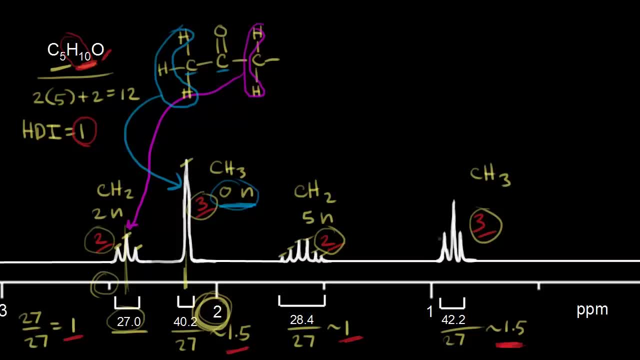 So that's a methyl group, So CH3.. How many neighbors? Well, we have one, two, three peaks, So three minus one is two. So we would expect two neighboring protons. Now, these two signals right, This signal here and this signal here. 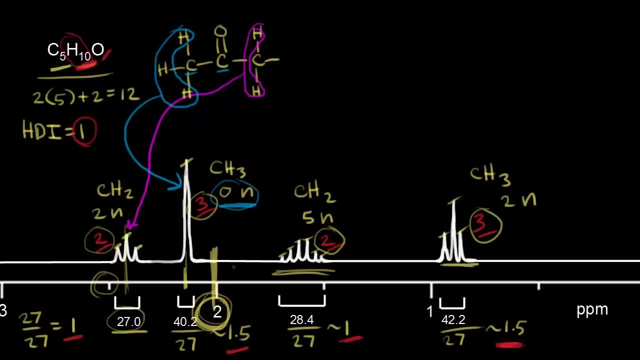 we're talking about under two parts per million now. So these must be further, the furthest away from the carbonyl right. So they're not being deshielded as much as the two signals in this direction. So these two neighboring protons for the methyl group. 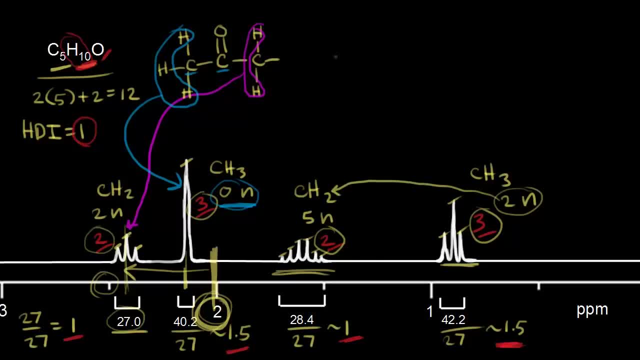 must be these two protons right here. So let's go ahead and draw that in. So we have our methyl protons right here And let me make these protons red. So these protons right here in red are giving us this signal. 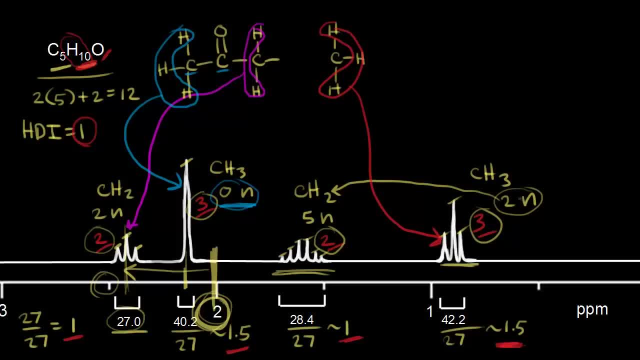 And from this signal we know that these methyl protons are next to two neighbors, And so we must have a CH2.. We must have a CH2 next to that methyl, And so let's go ahead and draw in our CH2.. 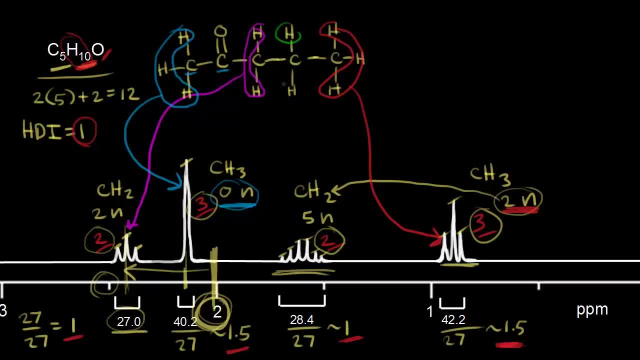 And this CH2 must be this signal right here. All right, so let's think about how many neighbors. We expected five neighbors for these CH2 protons. Let's count them up: One, two, three, four, five, So five neighboring protons. 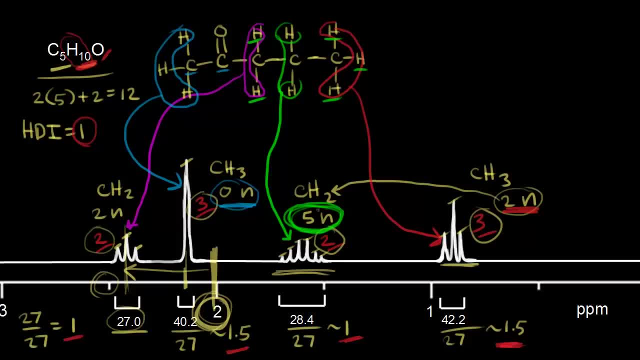 matches what we see on the NMR spectrum. Now, those protons, those magenta and red protons, are actually in different environments, And so the simplified version of the N plus one rule isn't quite true, but it works for this example. 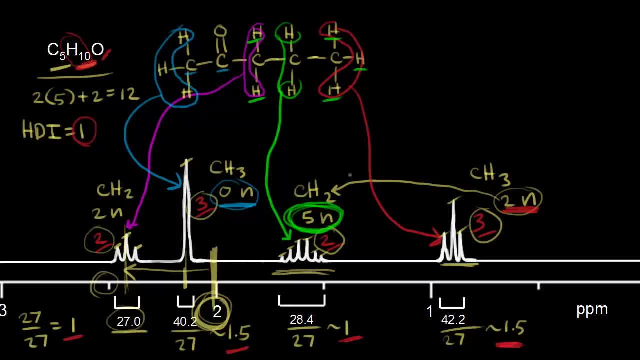 It works for this example, so we're gonna go with it, because all we care about is getting the structure of our molecule here, All right. so let's think about the red protons again. So the red protons are supposed to have two neighbors. 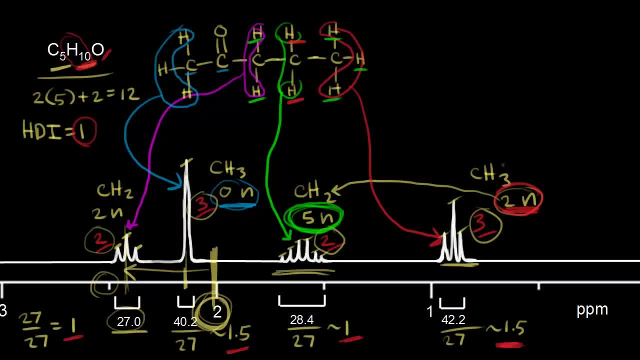 So how many neighbors do the red protons have? Here's one and here's two. So this makes sense. So that one makes sense. This one makes sense right here. We just talked about that. Let's think about the magenta protons. 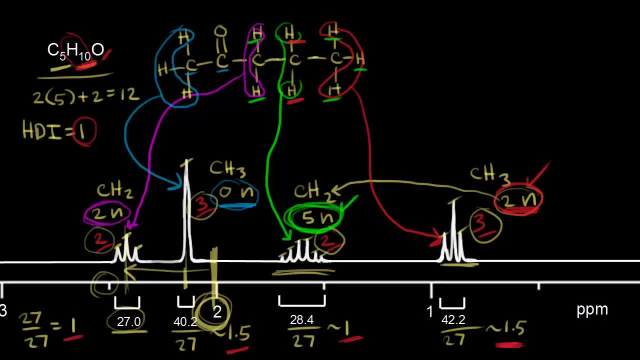 So the magenta protons were supposed to have two neighbors. So let's look at the carbon next door to this one. So here's the carbon next door. Here we have a neighbor, and here we have a neighbor. So this makes sense. 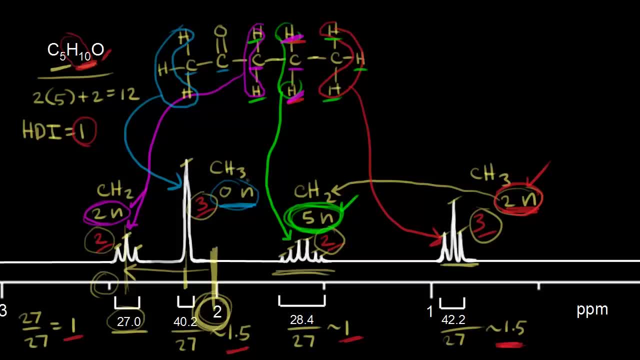 And then we already talked about the blue protons, right, Having zero neighbors. So everything seems to make sense here. And to sum everything up, make sure to count all of your atoms and you will get, of course, five carbons, ten hydrogens. 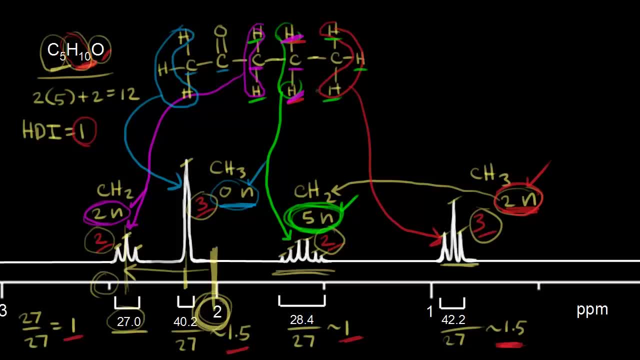 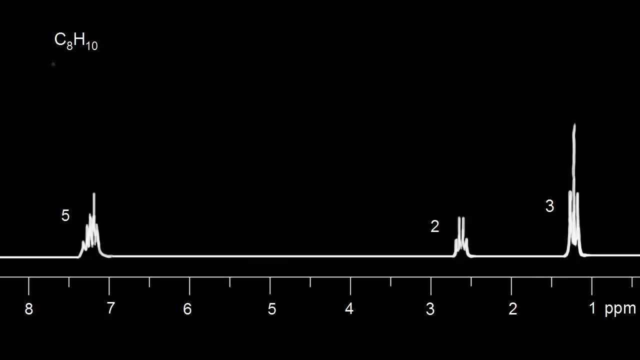 and one oxygen when you do that. So this is the dot structure that we were trying to find. Let's take a look at another one here. So we have a molecular formula of C8H10.. And let's go ahead and calculate the hydrogen deficiency index. So if we have eight carbons, then we can have a maximum of two times eight plus two hydrogens. So two times eight is sixteen plus two is eighteen. So for eight carbons eighteen hydrogens is the max. Here we have ten hydrogens. 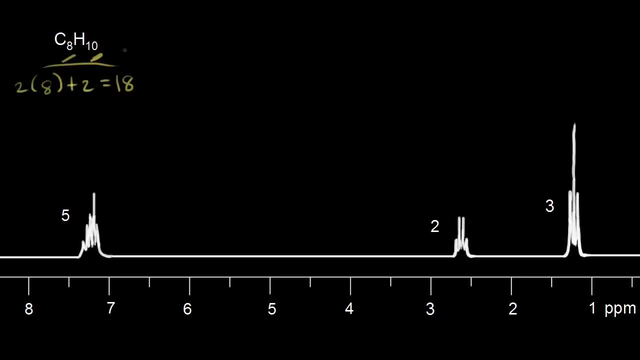 So we're missing eight hydrogens, or we're missing four pairs of hydrogens. So the hydrogen deficiency index is equal to four. Remember, any time your HDI is equal to four. you should think about a benzene ring. So I'm going to go ahead and draw. 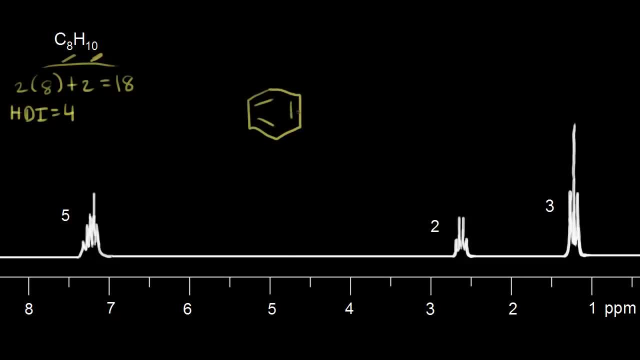 a benzene ring in here. And let's look at the integration. So sometimes you'll see the integration given like this: So this represents five protons for this very complex-looking signal right here. This signal over here represents two protons and this signal represents three protons. 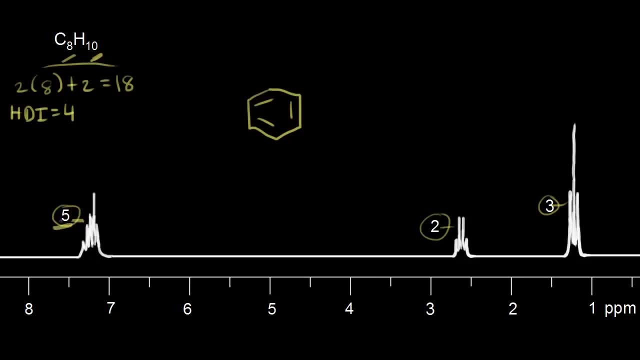 So let's go back to these five protons. with this complex signal. This is in the aromatic range, So approximately 6.528.. Those must be five aromatic protons. So we can go ahead and draw in five protons off of our benzene ring. 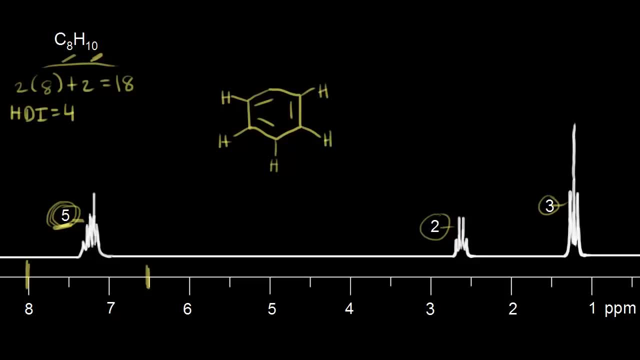 So, even though those protons are in slightly different environments, because this integration value is five here and we know a benzene ring is present, we're done. We don't have to worry about the slightly different environments. We know that these five protons 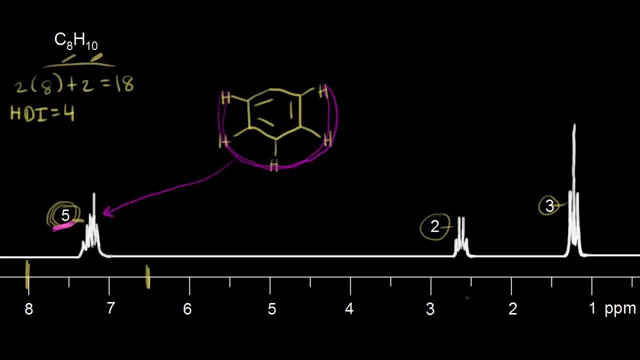 are giving us this complicated signal over here. All right, next let's look at this signal. So two protons, So that must be a CH2.. How many neighboring protons for this CH2?? Well, there's one, two, three, four peaks. 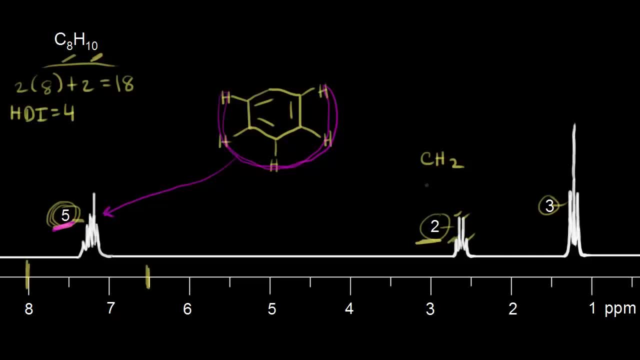 So if there's four peaks, four minus one is three. So these CH2 protons have three neighbors. All right, let's look at this next signal. So three protons, So this must be a CH3.. How many neighboring protons do we have? 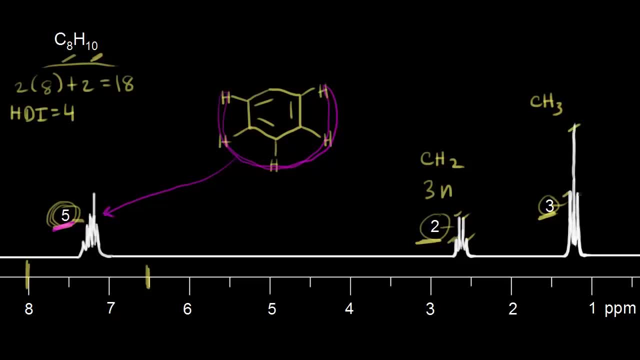 for the CH3 protons. Well, we have one, two, three peaks, So three peaks. three minus one is two, So two neighbors, And so two neighboring protons. that must be these two neighboring protons, And so we can go ahead and draw an ethyl group. 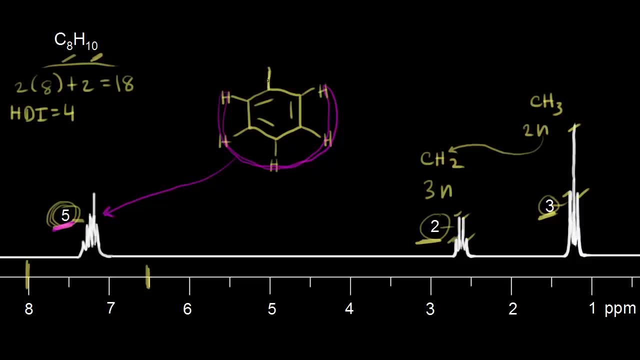 So this is an ethyl group pattern over here. So there's a CH2, and there's your CH3.. So let's draw in all of our protons. So we have these protons, and we have these protons, And let's color coordinate here. 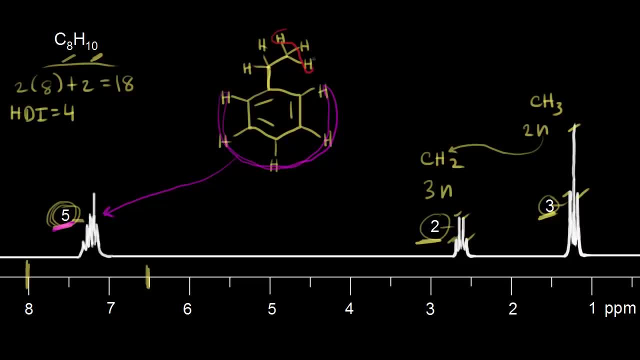 just to make sure everything makes sense. So these red protons: right here, they must be giving us this signal. So these methyl protons: right, We'd expect two neighbors, because we have three peaks on our signal. And here are the two neighbors. 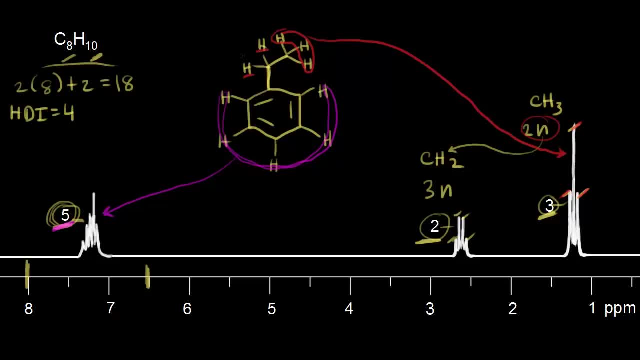 One, two, so two neighboring protons. Let's look at these two protons next. So these two protons are giving us this signal. We would expect three neighbors, because we have four peaks: One, two, three, four, So three neighbors. 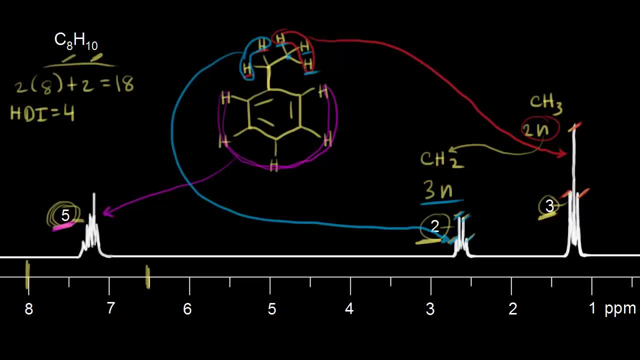 So here's a next-door carbon, So one, two, three, three protons. And then this is also a next-door carbon, but there are no protons on this carbon, And so we see only these three neighbors, And so everything seems to make sense. 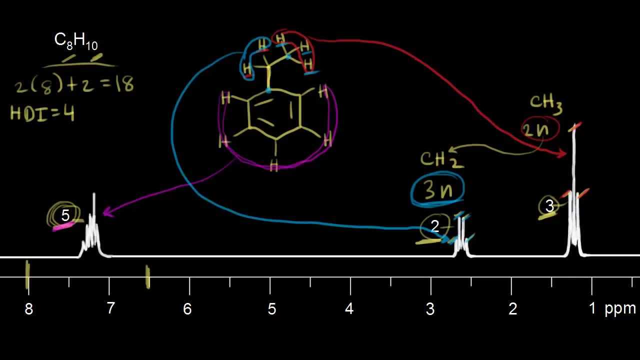 And once again count up all of your atoms and make sure you've accounted for everything. For example, you have eight carbons You have to worry about. So on your ring we know there are six, One, two, three, four, five, six.